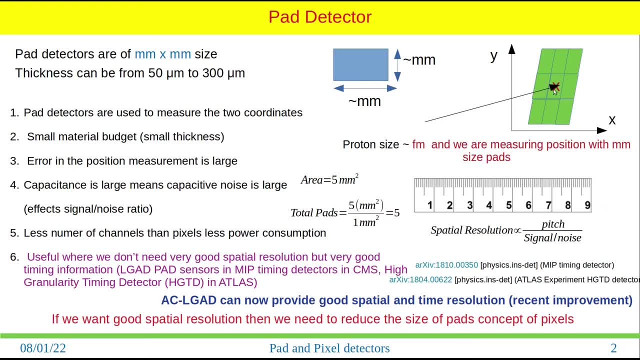 detectors are used to measure the two coordinates. when, suppose, this pad is fired and the position of the particle is given by the center position along the x direction and the y direction and we have the small material budget because we have the small thickness and the error in the position, measurement is. 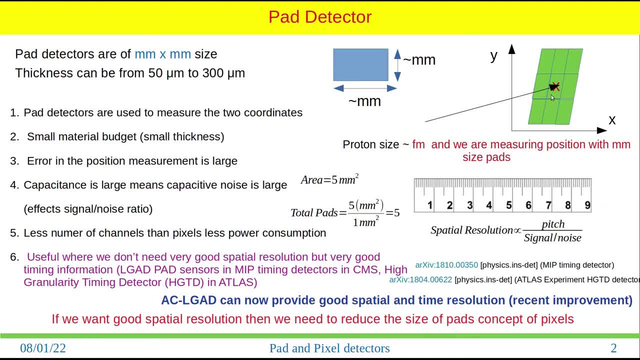 large because the size of the pads are large, like mm- typically of millimeter, and the capacitance is large because your area is large here, and then you have a large capacitive noise and then that can decrease, that can decrease a signal to noise ratio and then if you have this number is small, then you have 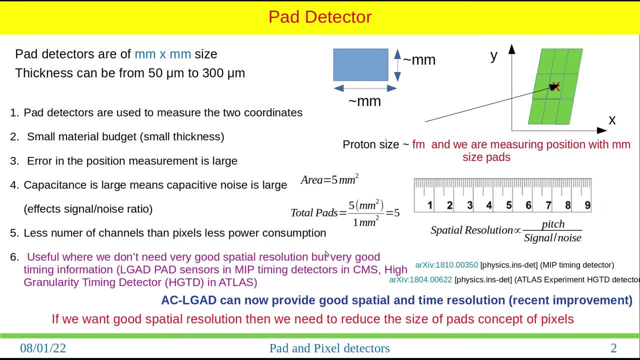 the large uncertainty in the measurement of the position, and here we have a less number of channels than the pixels, so we have a less power consumption. suppose we have the active area of five millimeter square and then then we have a one millimeter by one millimeter pair, then we have a power consumption of five. 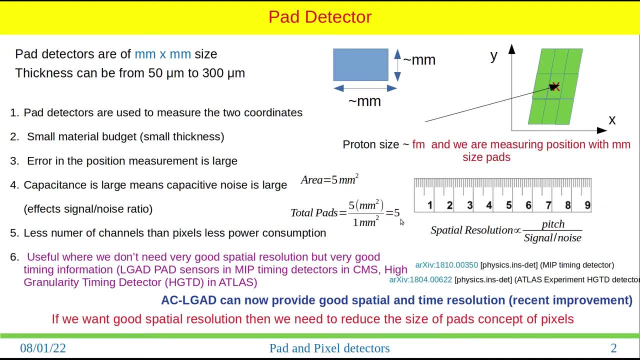 millimeters and then then we have only five pets. that means we have only five channels. these are useful when we don't want a good spatial resolution because we have a large size bed and but we want a very good timing information. so these are used, used in the CMS experiment and I'll get. pet sensors are used in CMS. 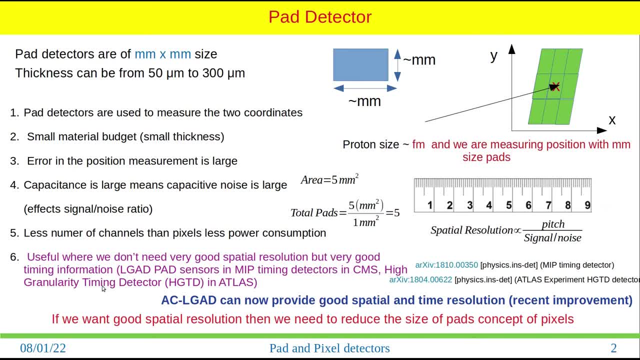 experiment at IMIP timing detectors and a high granularity timing detectors in the in the atlas experiment. now, in the recent improvement, the ACL gets technology also developed which can provide the good spatial resolution as well as the timing resolution. if we want good spatial resolution, then what we have to do, since we have to reduce the 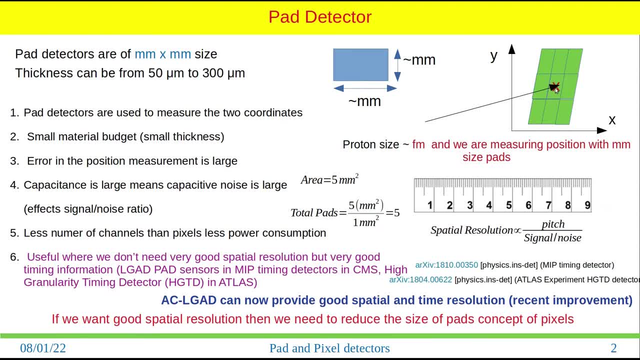 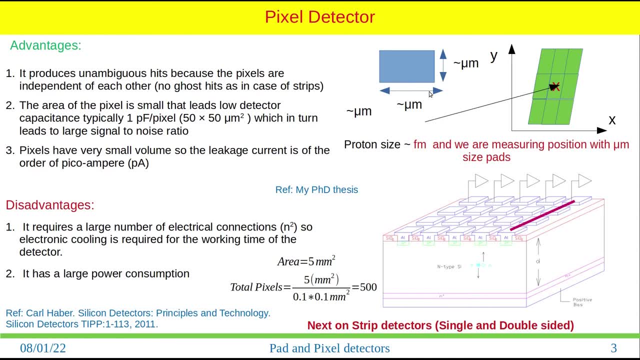 size of the pads. basically, there it comes to the size of the pixels, which are smaller in size. so pixels are typically of the of the micrometer square area sensors, so we can use many pixels to measure the position, as I explained before. so in the reality these, we have many pixels on the buffer, so you can see. 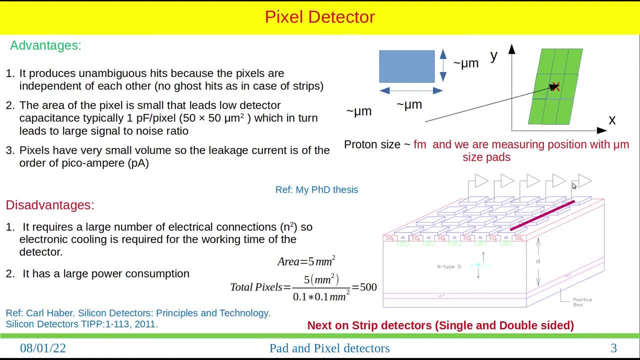 that these are created by photoregulatography method and each pixels we have a. we can read the signal, so we have a channel for each pixel. so these are the curve. this is the configuration. so pics. there are several advantages of using the pixels. it produces a very good spatial resolution and we can see that. 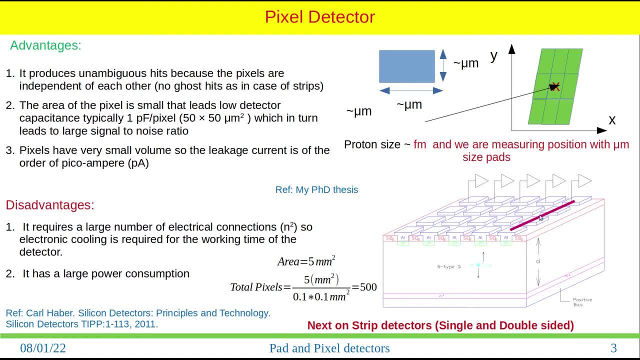 by the way of this pixel resolution, which produces an ambiguous hits, because pixels are independent and we don't have any issue of goal sheets, which is basically in the case of strips, which I will explain in my next video- and the idea pixel is small because your idea is small and so your capacitance is small. 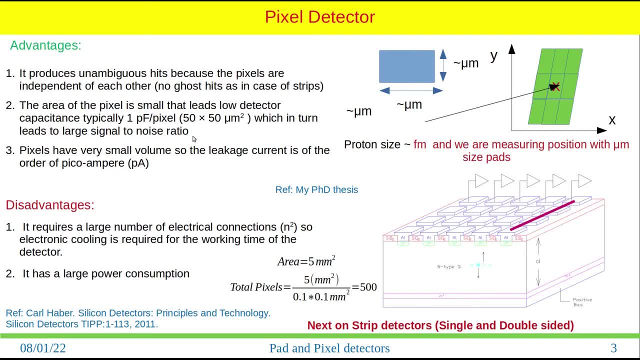 and capacitance is in for small means. capacitive noise is small, which will improve your signal-to-noise ratio and that will improve your spatial resolution again. and pixels have very small volume and so we have a small leakage current, typically of the order of pico ampere, and the disadvantage of you have a larger electrical connection. 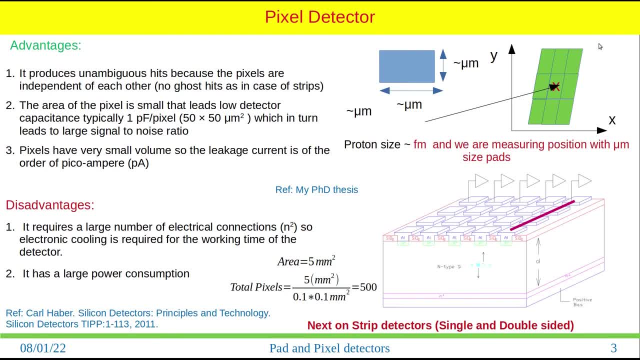 suppose you have n pixels in the directions and pixel is in this directions, then you have the total pixels, n square. so that corresponds to any square connections. so we have a large connections here. so electronic cooling is required, required for the parking of the detector, and it required. 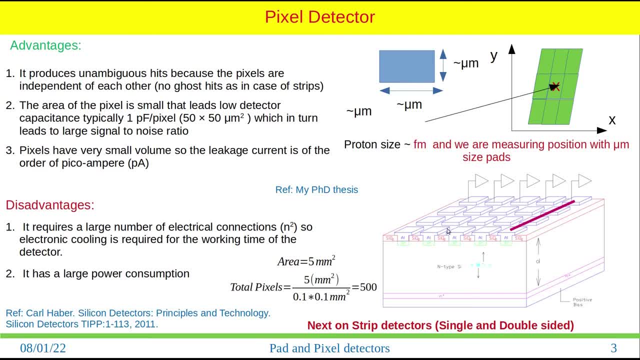 large power consumption because we have a large number of pixels and any square pixels for an area. suppose in the previous example, as I mentioned, that let's assume the area is again 5 millimeter squares and the typically pixel size is assumed that's 100 micrometer. 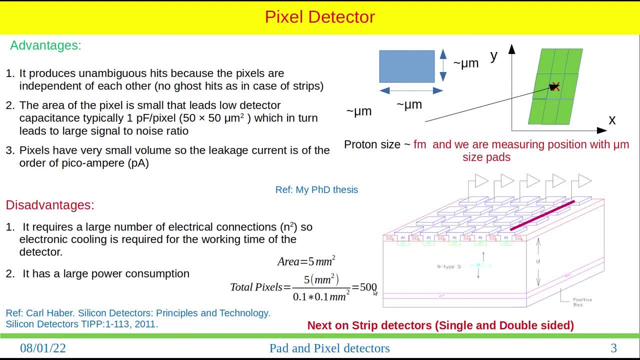 by 100 micrometer, then you have a 500 pixels here, while you have only five pairs here. so you have 100 times more channels here. so that's just a disadvantage of using the pixel. so we have a large number of channels and large power consumption. typical size of the pixels we use of the 10 micrometer by 10. 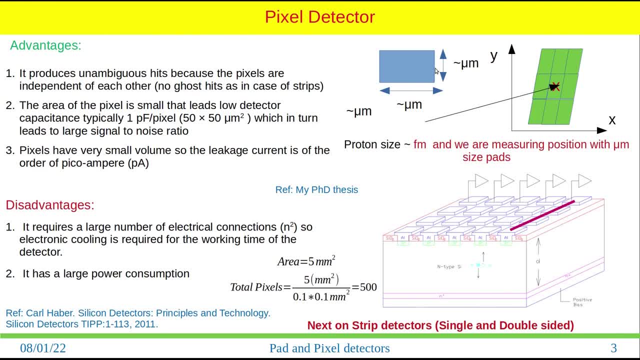 micrometer in the future, but currently people are using, in high energy physics, 50 micrometer by 100 micrometer, 50 micrometer by 50 micrometer pixels, so neck. in my next video I will explain about more details about the strip detectors, single-sided, as well as. 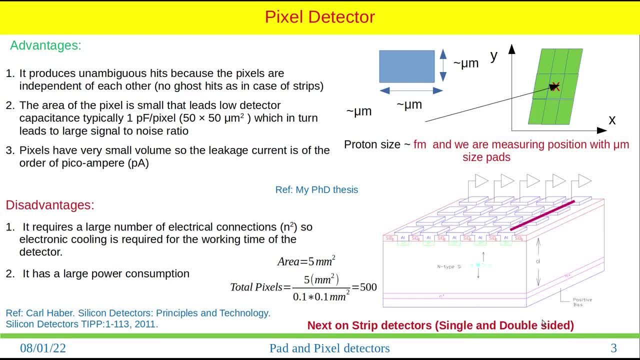 double-sided detectors, and what are the advantages and disadvantages where we have to use these types of configuration? this configuration is also used by many, many experiments, so I will give a more detailed about it in my next video. okay, thank you.